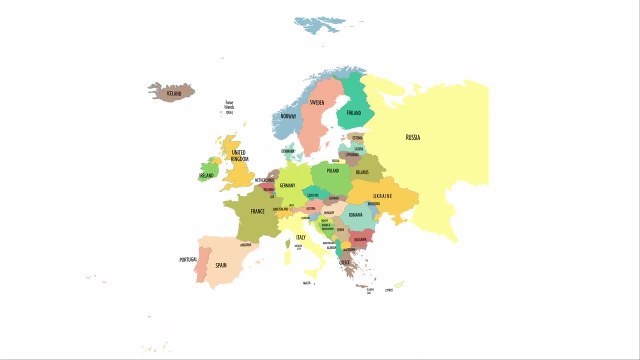 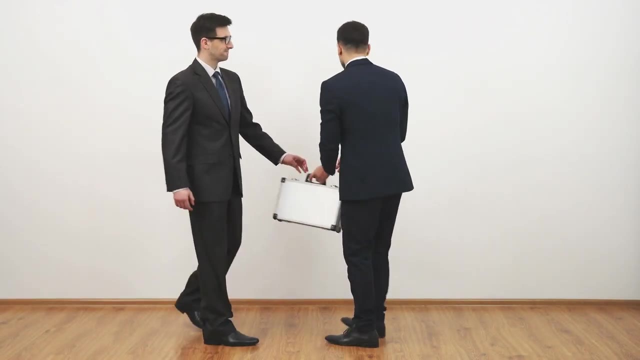 soil Crops were being taken back to Europe as well, like corn and potatoes. This exchange of both plant and animal life ended up being very beneficial to both sides of the exchange, But sometimes, when flora and fauna are moved to different ecosystems, the results can be quite disastrous. In 1876, the kudzu plant, native to Japan and southeast China, was brought to the United States as part of the Philadelphia Centennial Exposition, where it was touted as a great ornamental plant for its sweet-smelling blooms. 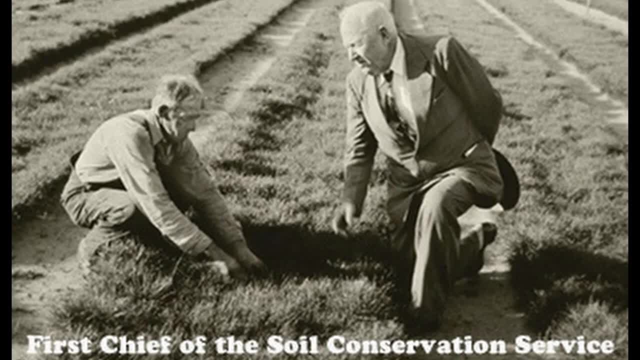 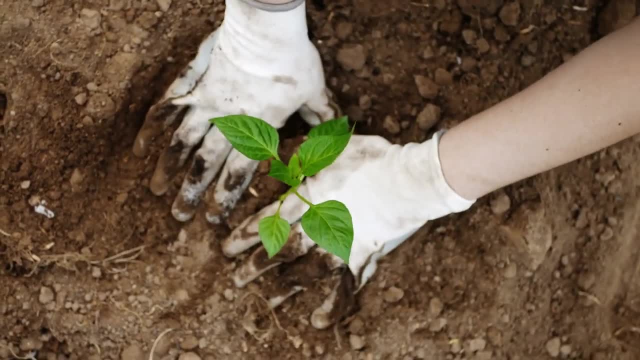 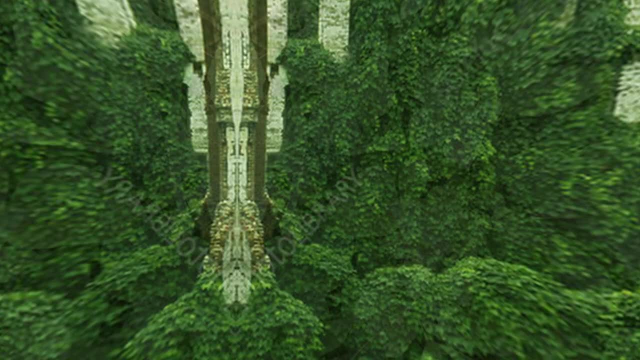 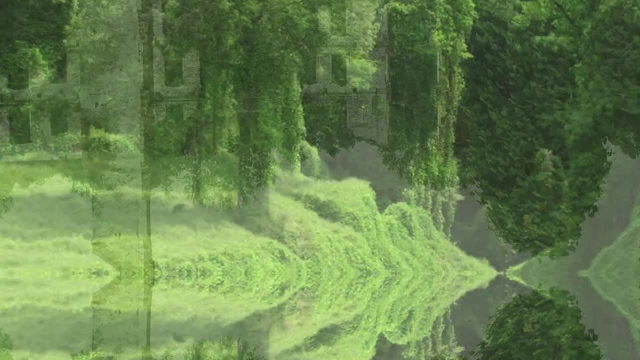 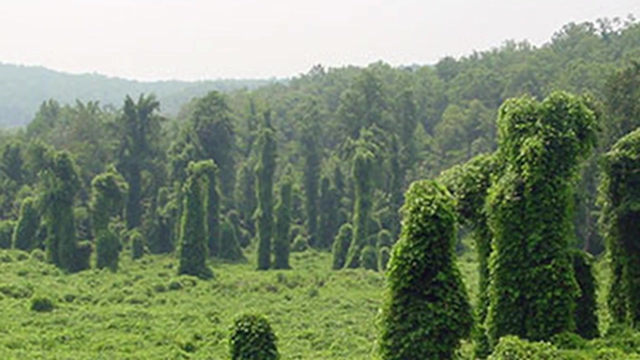 left unchecked by any form of natural predator can get out of control very quickly. It grows over a foot per day, with 30 vines coming from one root system and getting up to 100 feet long at maturity. It grows quickly, overtaking and encasing anything in its path- An invasive plant. 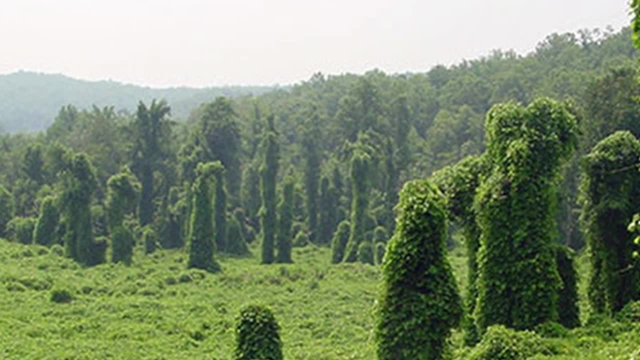 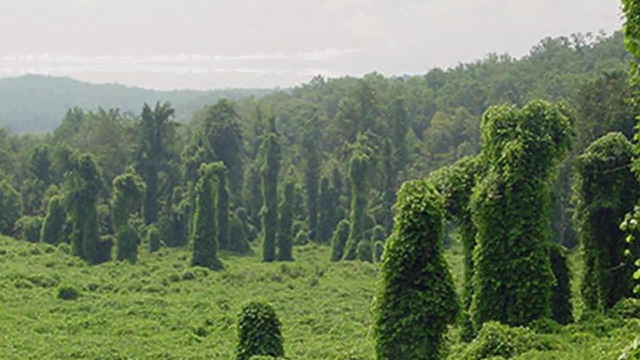 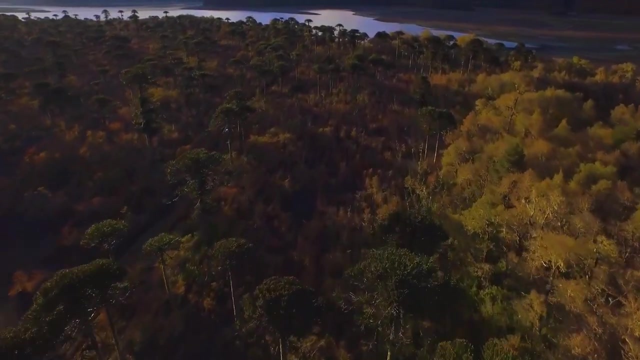 as fast-growing as kudzu out-competes everything from native grasses to fully mature trees. The loss of native plants can harm other plants, insects and animals that have adapted alongside them, leading to a cascading effect through the ecosystem. Over time, these effects of habitat loss can lead to the extinction of species. 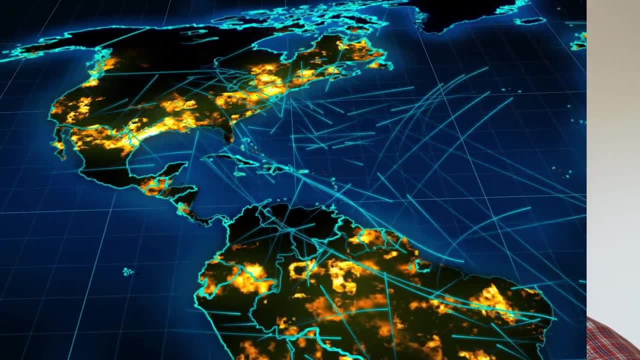 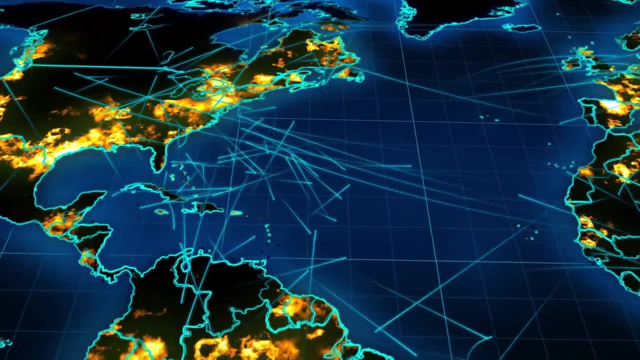 But what makes a species invasive? An invasive species is an organism that is not indigenous or native to a particular area. They can cause great economic and environmental harm to the new area. Not all non-native species are invasive, however. As I mentioned earlier, most of the food crops grown in the United States, including popular varieties of wheat, tomatoes and rice, are not native to the region. To be invasive, several boxes must be checked, While all species must compete to survive. invasive species tend to have similar characteristics that allow them to succeed in environments they didn't evolve in. In fact, 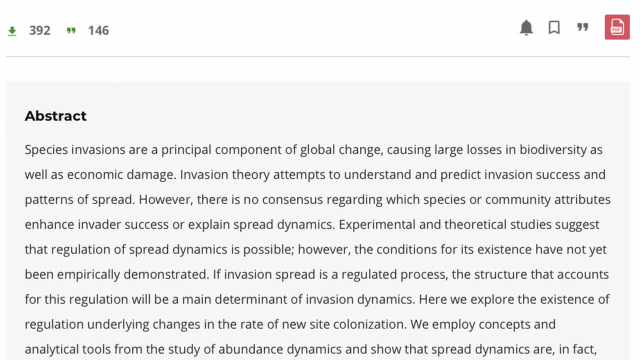 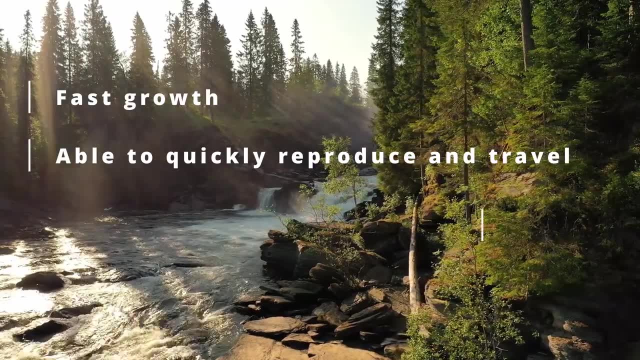 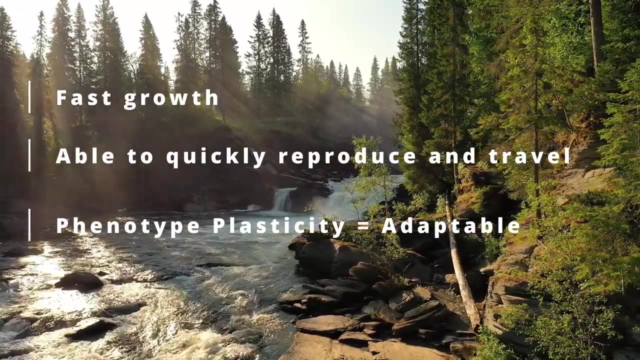 one study found that 86% of invasive species could be identified from their traits alone. These include fast growth, rapid reproduction, high dispersal ability, phenotype plasticity, tolerance of a wide range of environmental conditions, ability to live off a wide range. 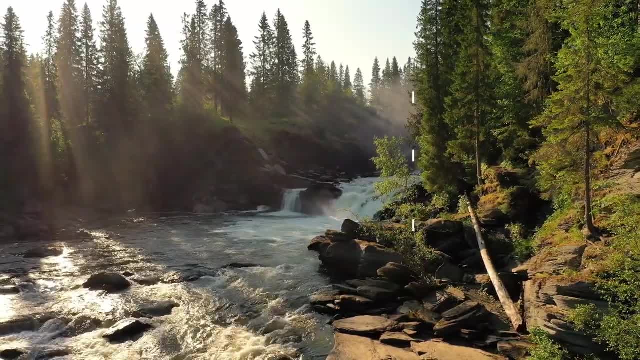 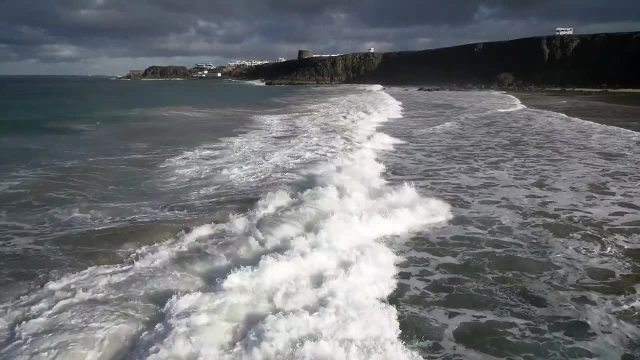 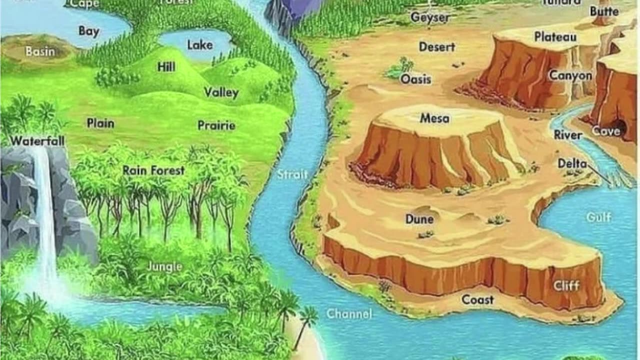 of food types and association with humans, as humans tend to be the number one factor for transmitting invasive species to new environments. In the past, oceans, rivers, mountain ranges, deserts and other geographic features provided barriers that limited the spread of species from one place to another. Humans, with our cars, boats and airplanes, have made 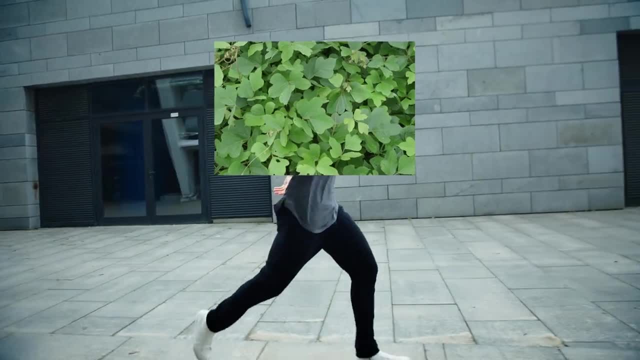 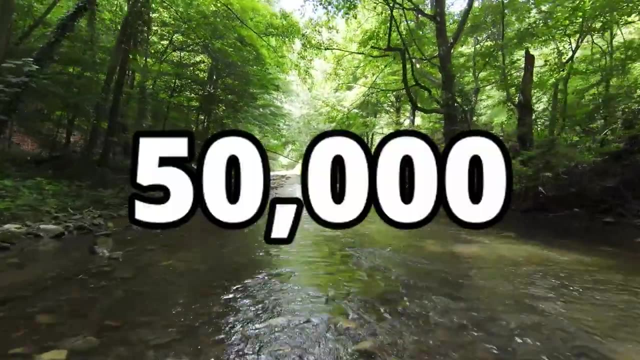 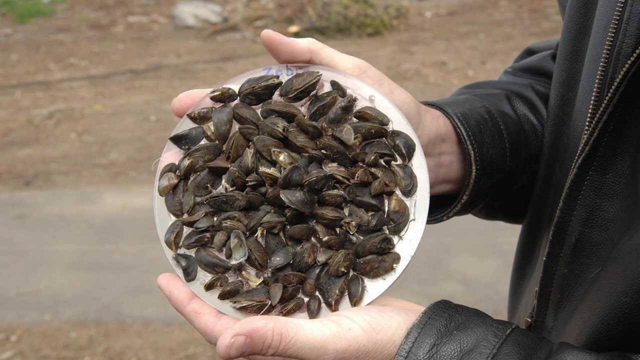 these natural barriers meaningless. As a result, plant and animal species can move rather quickly from one area to another. Scientists now estimate that there are 50,000 non-native species in the United States. Some of these spread by attaching to the bottoms of boats. That's how we got the 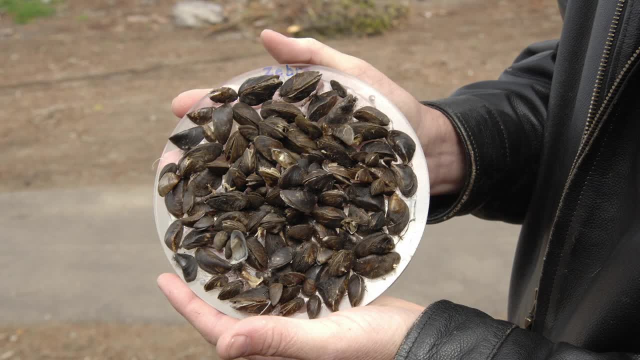 zebra mussel into the Great Lakes from Europe. The mussels are so resilient and so invasive that they eat the food they usually eat. The mussels are so resilient and so invasive that they eat the food they usually eat. The mussels are so resilient and so invasive that they eat the food they usually. 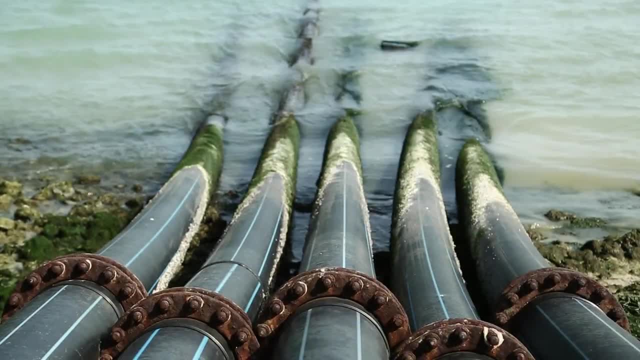 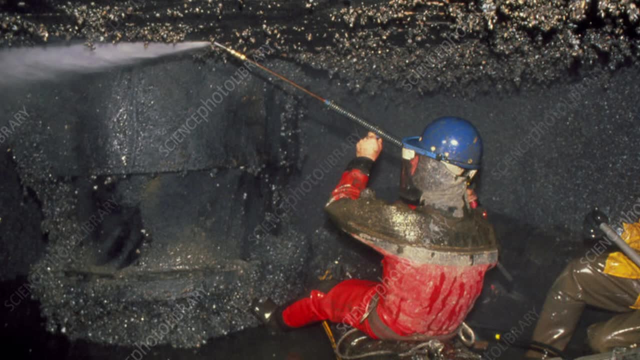 reserve for the native species of fish. When they enter a body of water, they can clog water intake pipes, disrupt cooling systems in boat engines and have even damaged water pipes at power plants in the Great Lakes area, not to mention their ability to muscle out native species in the region. 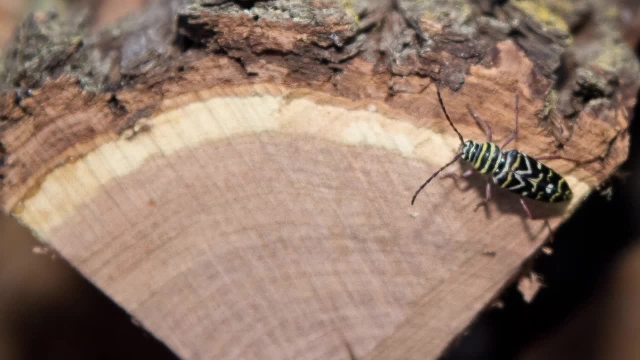 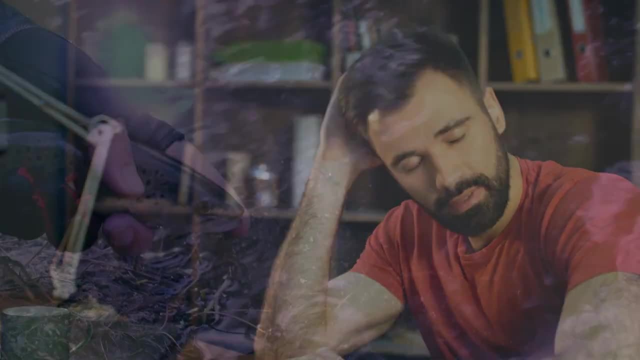 Invasive insects can move from area to area by boring into firewood, shipping pallets and other products, And sometimes humans release killer species into the environment on purpose. Hunters, fishermen and those in the wild have a hard time managing the environment. They are often 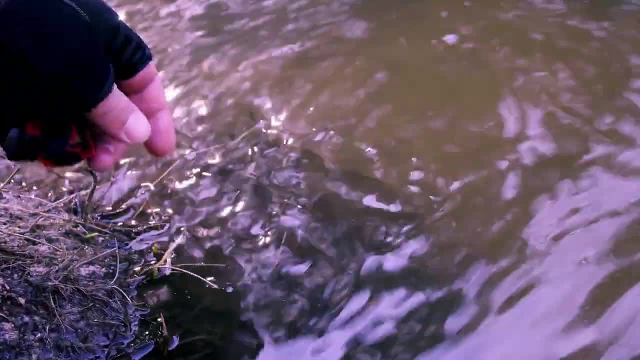 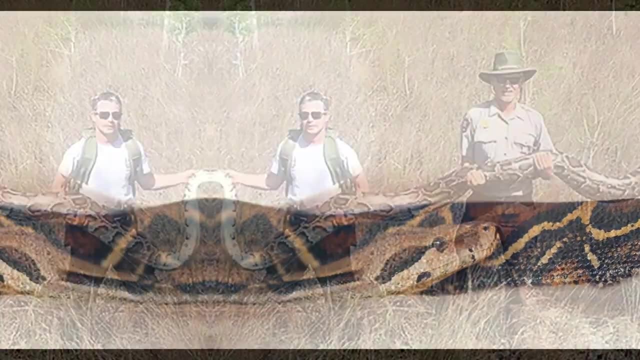 the pet trade often release non-native animals for one reason or another. For example, many people have released pet Burmese pythons into the Everglades Swamp in South Florida. These huge snakes can grow up to 20 feet long. Originally native to the jungles of Southeast Asia, the 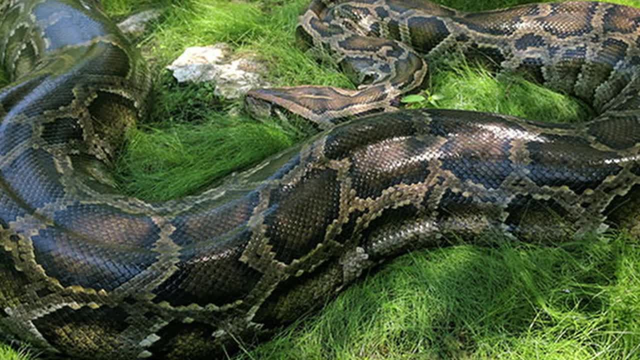 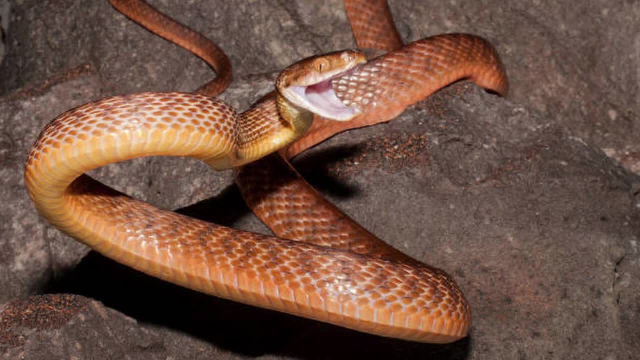 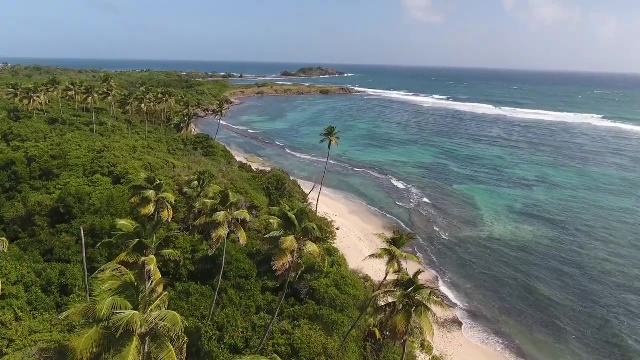 Burmese python has few predators in the Everglades and thus feast on many of the unsuspecting local species. Continuing with snakes, brown tree snakes were accidentally brought to Guam in the late 1940s, and the island was full of birds, rodents and other small animals they liked to hunt. 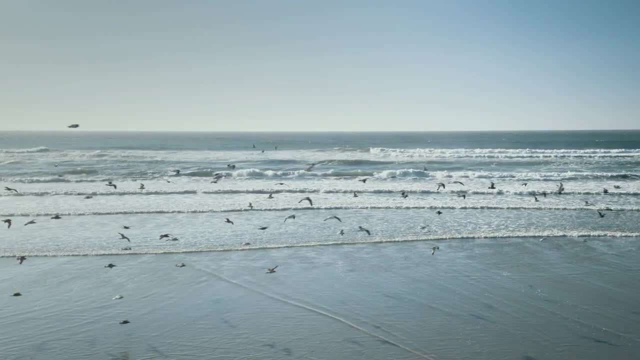 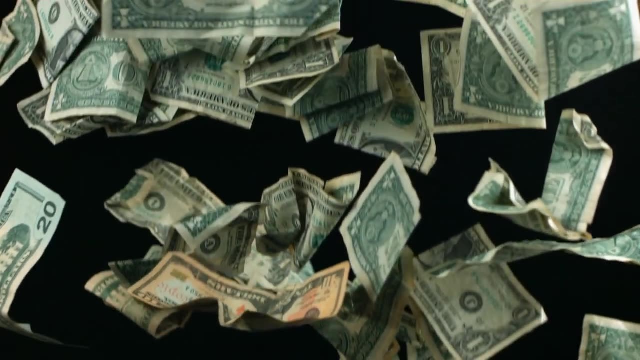 the snakes quickly multiplied and are considered to be responsible for the extinction of nine of the island's eleven forest-dwelling bird species. Much like the zebra mussel, invasive species have a very clear monetary impact. The water hyacinth is a plant native to South America that has become 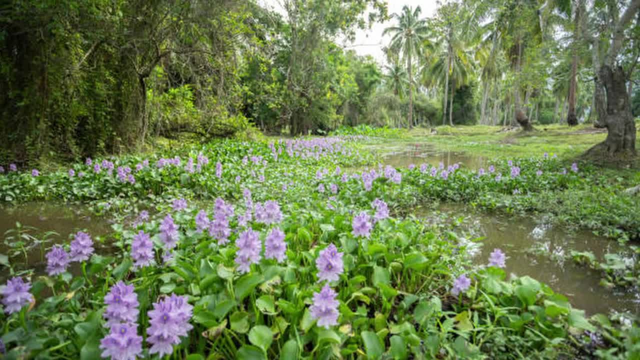 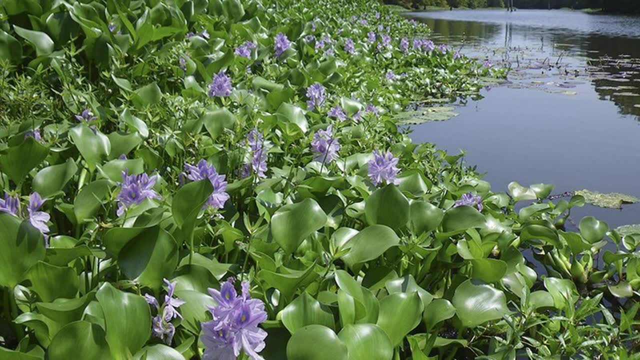 an invasive species in many parts of the world. People often introduce the plant, which grows quickly in the water, because of its pretty flowers during bloom, But as it spreads, it can quickly overtake everything around it, choking out the local wildlife and causing fishing industries to decline. 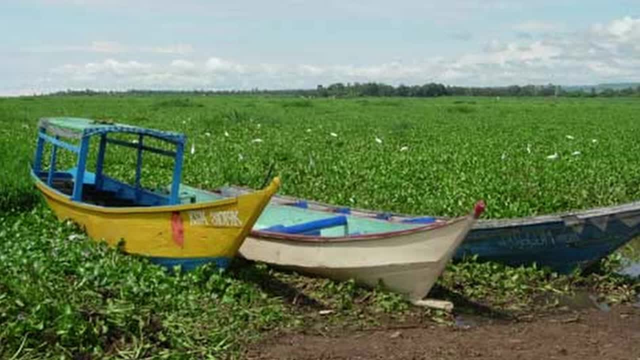 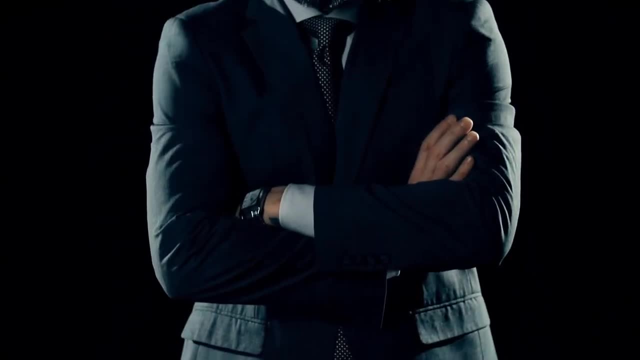 In Lake Victoria, Uganda. they grew so thickly that boats could not get through, causing some ports to close down. So what's being done about the invasive species once they are discovered? Well, in the 1970s, fish farmers in the southern United States imported Asian carp, but one. 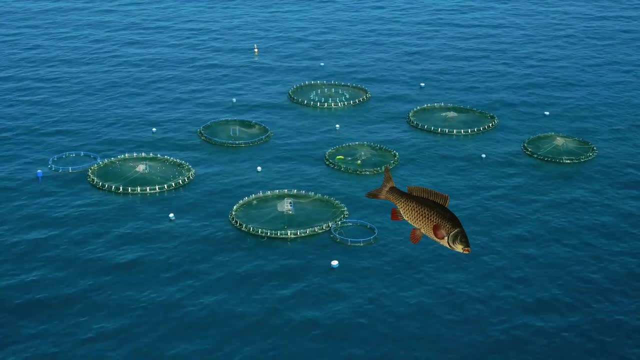 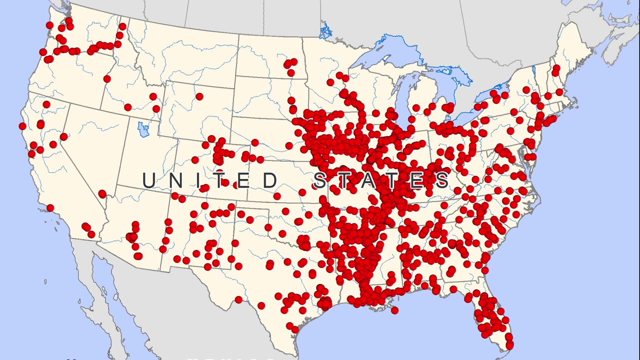 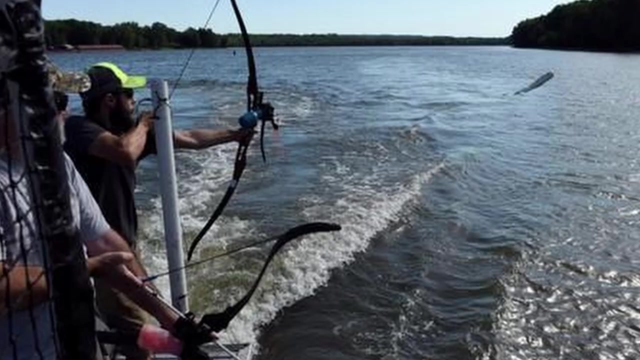 day the carp made a break for it and escaped into the Mississippi River. Now the Asian carp swims in the waters of at least 23 states, destroying the biodiversity in many bodies of water. How do you kill the fish? Well, the US Geological Survey has developed a poison, but some fishermen just go out and 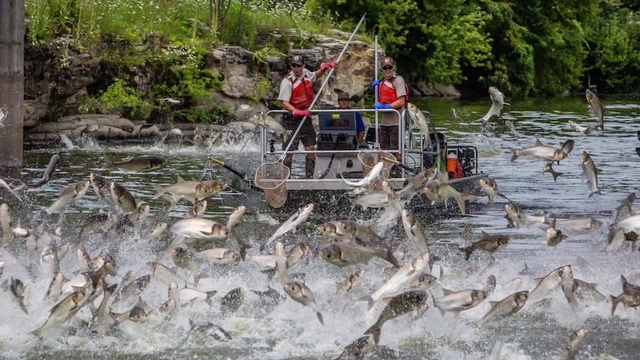 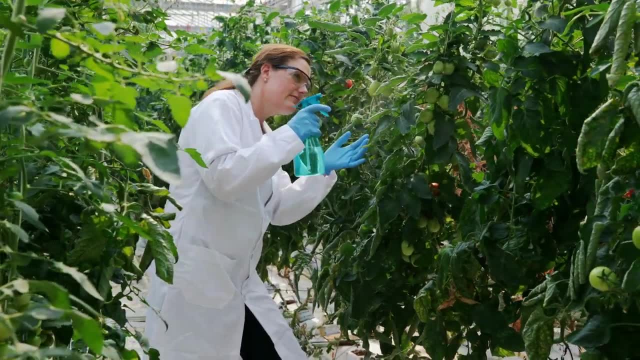 shoot them with arrows as they jump out of the water. Others, however, are catching the carp and eating them. They say it tastes similar to tilapia. Dealing with the Asian carp reflects on the problems humans face when trying to control or eradicate any invasive species. 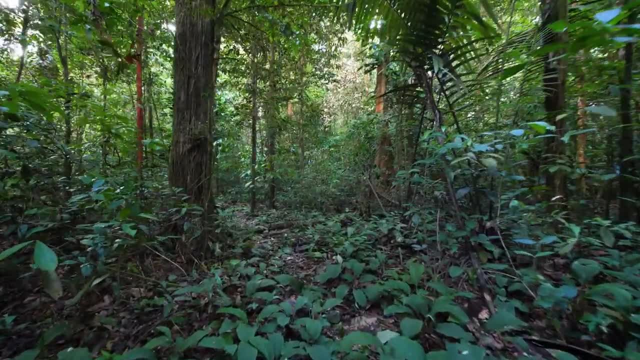 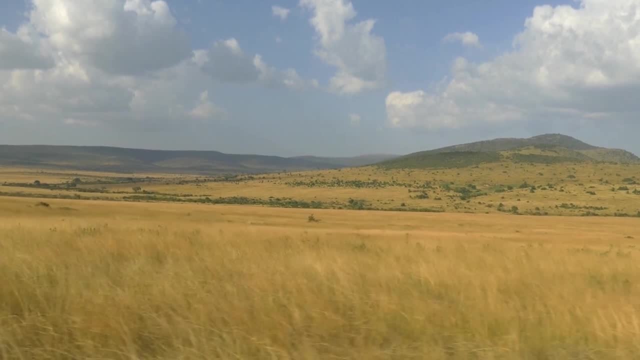 You would think that killing these fish would be easy. But what is it? You would think that killing these fish would be easy, But what is it? These pests would be an easy thing, especially when considering that when a non-native species enters a new ecosystem, only about 10% of the population will survive. 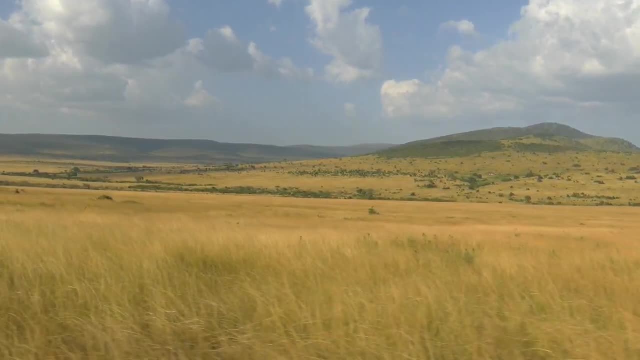 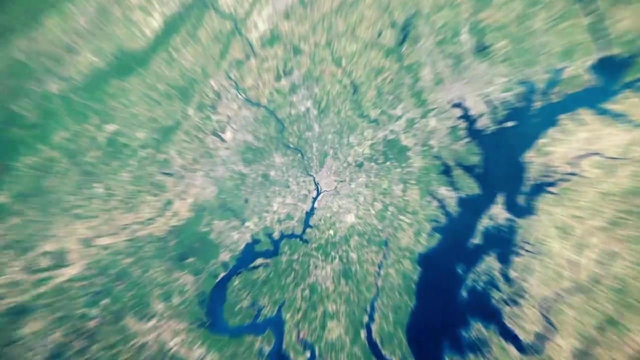 And of those survivors, only about 10% become pests. So what's the problem? At first, all infestation is localized. In fact, it's so local that humans don't even know it's occurring. Eventually, the species breathes and gradually moves into other areas. 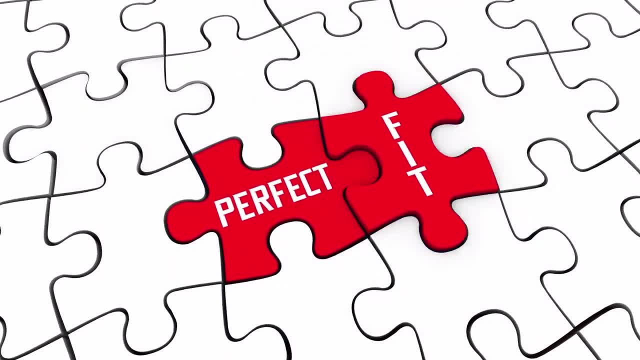 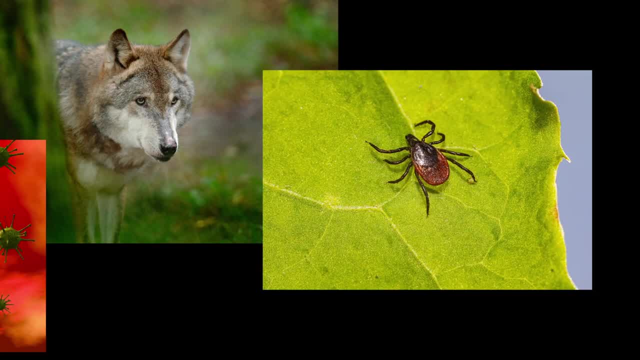 However, the climate has to be just right and the conditions have to be perfect for an invasive species to take over a new area. That means the area has to lack natural enemies, including parasites, predators or pathogens. Some species, such as aphids, spread more easily than others because a male is not required. 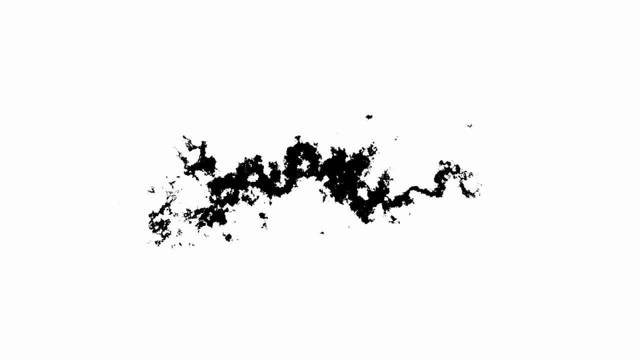 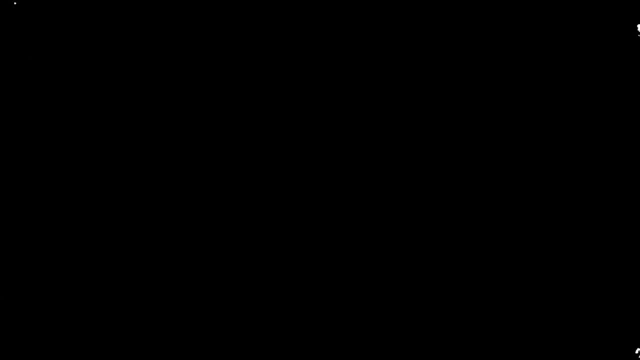 for fertilization. By the time humans figure out an invasive species has taken over an area, it's usually too late to easily do anything about it, But we try to anyway. There are two main ways of controlling an invasive species. The first is something researchers call proactive breeding. 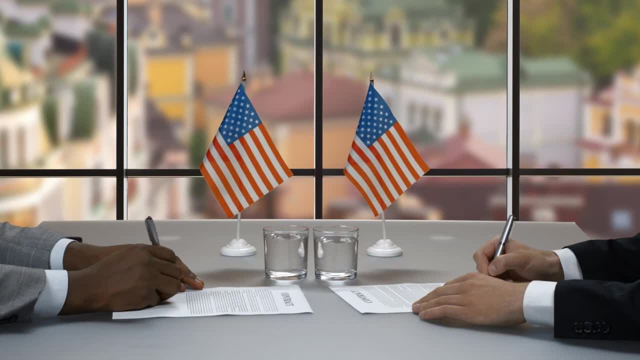 The first is something researchers call proactive breeding. The first is something researchers call proactive breeding. The second is something researchers call proactive management. That means excluding species by passing laws banning certain animals, plants, food and other products from coming into a country. 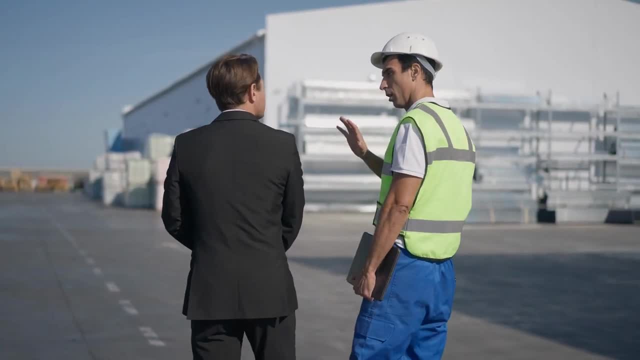 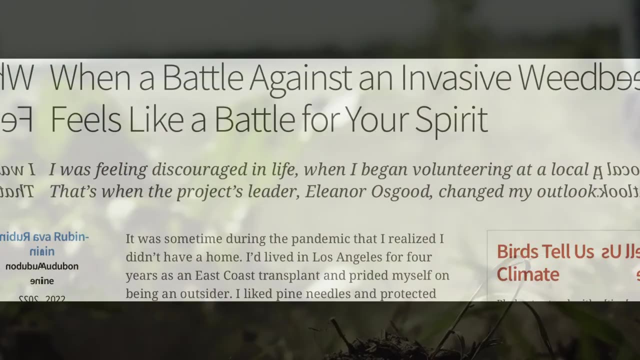 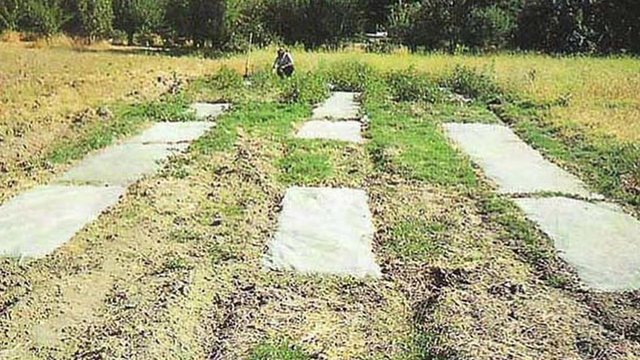 Officials can catch many invasive species by stepping up border inspections. Proactive management also means destroying an invasive population during the early stages of infestation. In California, environmental officials successfully beat back an invasive weed that can occur in tropical waters. When state officials spotted the plant, they shrouded it with tarpaulins and poured chlorine. 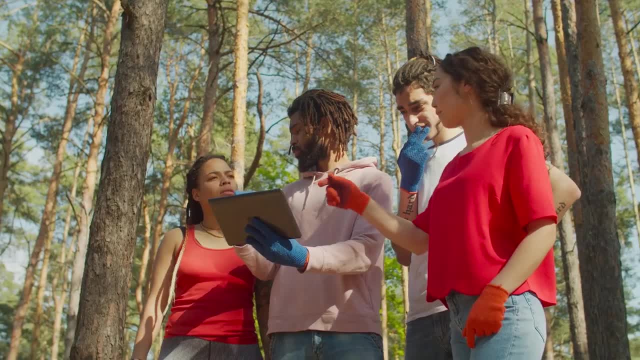 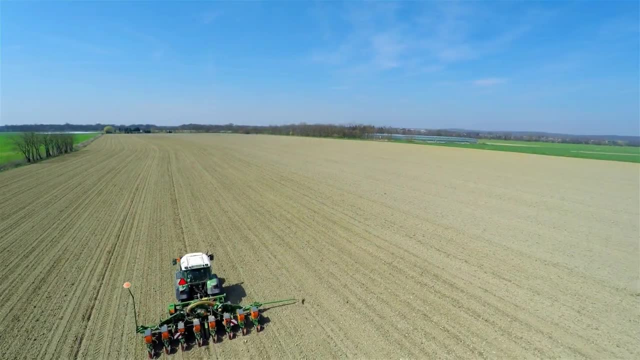 on top, killing the weed before it had a chance to spread. The second way to control an invasive species is through reactive management. That could mean doing nothing, Or it could mean controlling the invaders by limiting their capacity to reproduce. This could mean planting crops that are resistant to a plant disease. 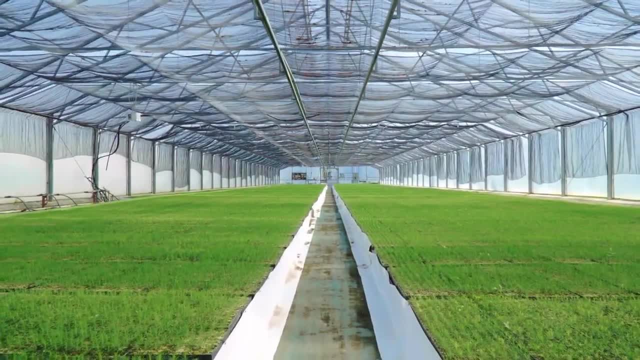 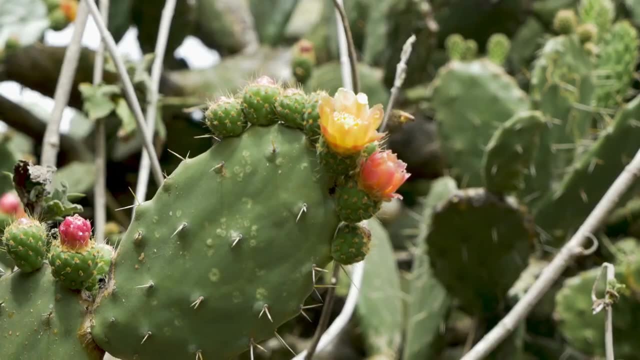 Or it could mean planting during a time of the year when pests aren't around, Or we could fight nature with nature and introduce another species to act as a predator. In Australia, the prickly pear cactus, which is native to the Americas, was growing out of control. 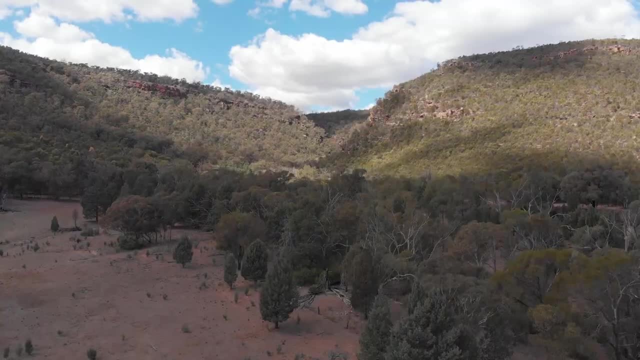 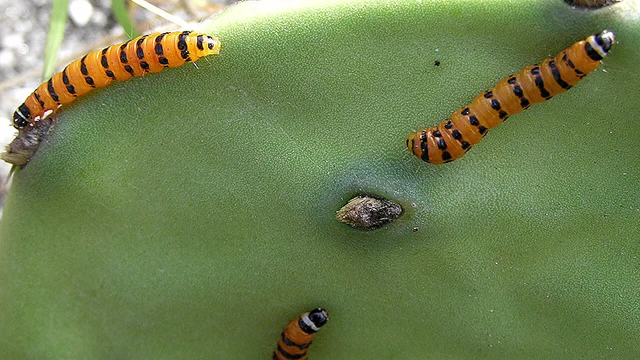 The cactus was destroying rangeland where ranchers raised livestock, So the government brought in cactus moth caterpillars to eat the cactuses, acting as a natural predator. Introducing other species can be dangerous. however. Sometimes they also damage a different species. 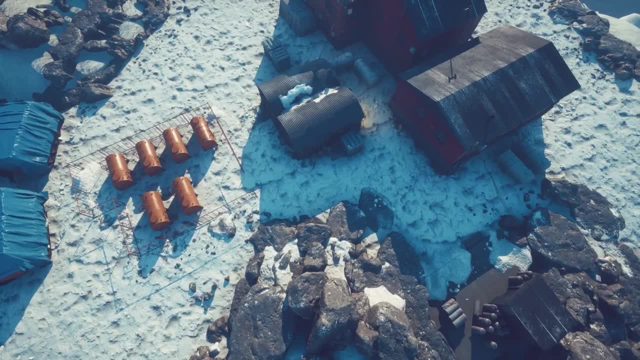 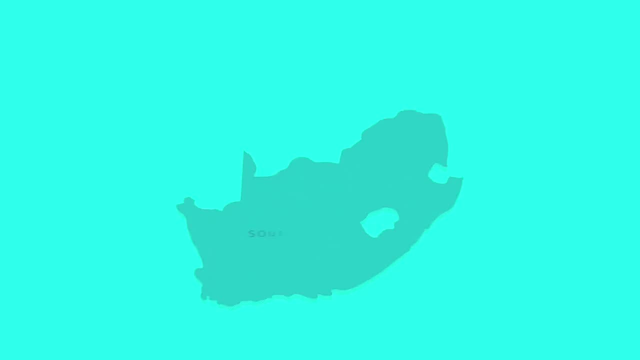 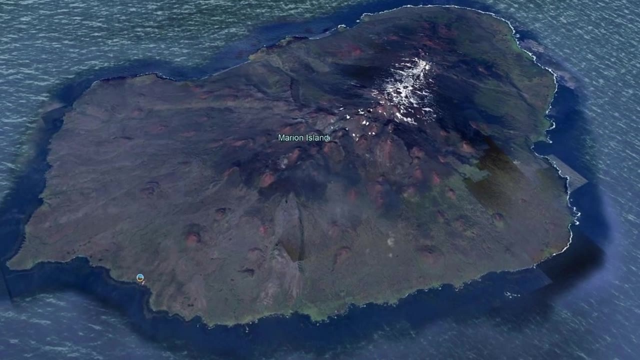 becoming an invasive species themselves. On a small island in the sub-Antarctic region, a research station was built and a problem was born. The island had been claimed by South Africa in 1947, and the research station was established on Marion Island soon after. 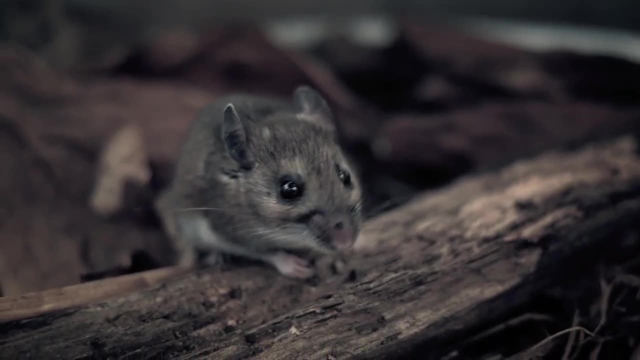 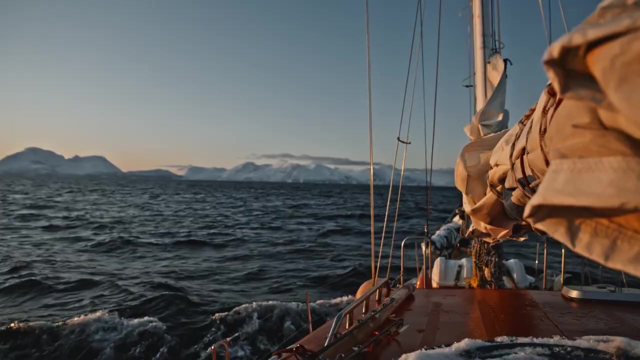 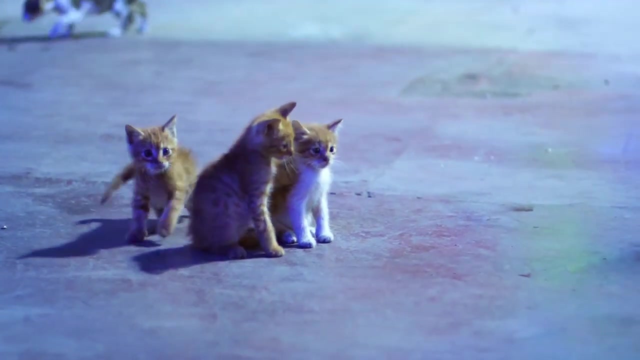 The buildings almost immediately began suffering from a severe mouse infestation, some of which may have snuck onto the island on the vessels that the researchers themselves had arrived on, And so a simple solution was adopted: In 1949, five domestic cats were imported to take care of the unwanted pests. But nobody neutered the animals. The consequences were disastrous. Within 30 years those five cats turned into 3,500 feral cats on the 12 mile by 7 mile island. The thousands of cats quickly began turning their attention from the mice.